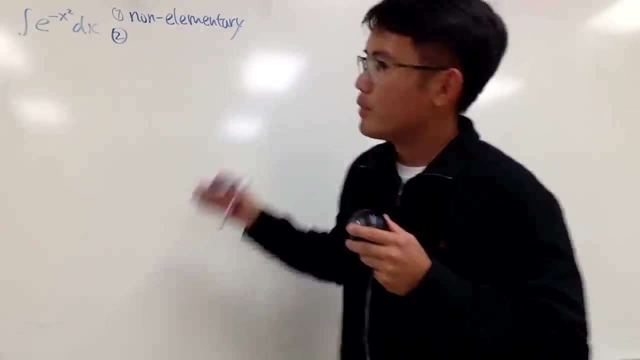 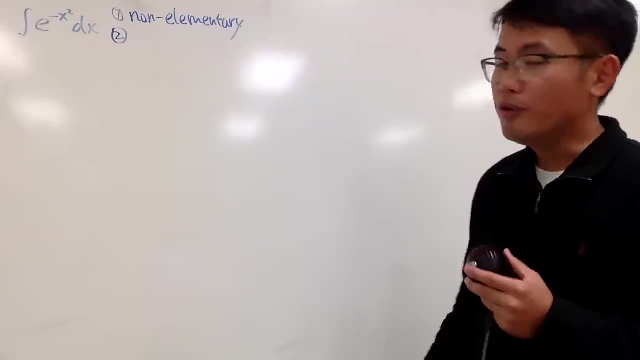 I don't want that to happen. So the second way to deal with this is that we can invent some new functions so we can continue our study, And the new function that we're going to use is what we call the error function, And the abbreviation is erf of x. 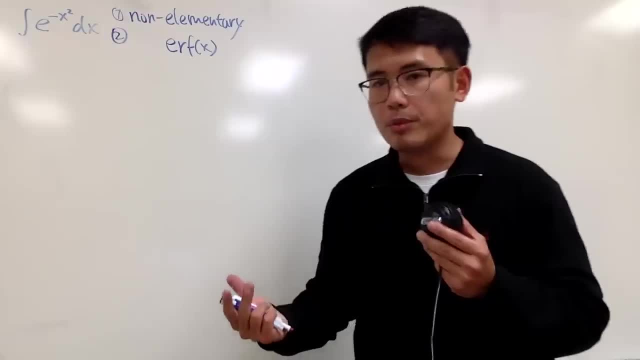 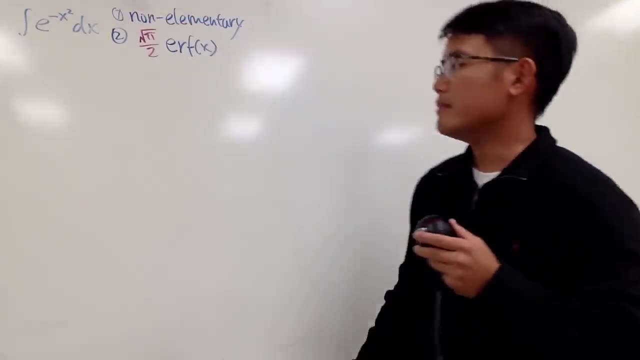 But not quite. There is actually some constant multiple in front. And what's a constant multiple? It's, right here, square root of pi over 2.. And you might be wondering: why is this the case? And now let's talk about this in detail. 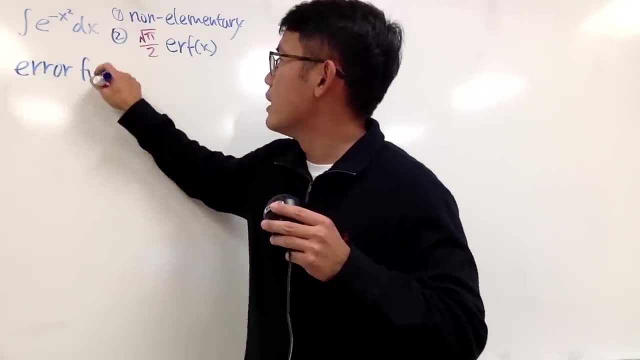 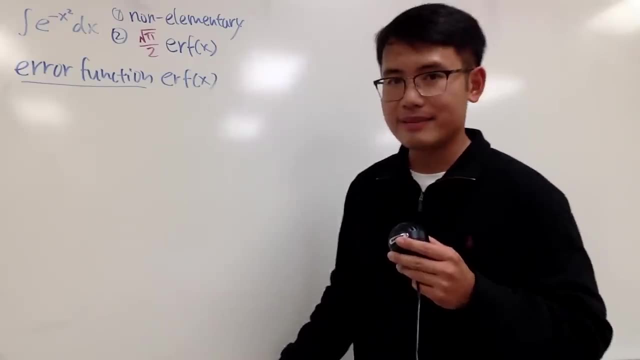 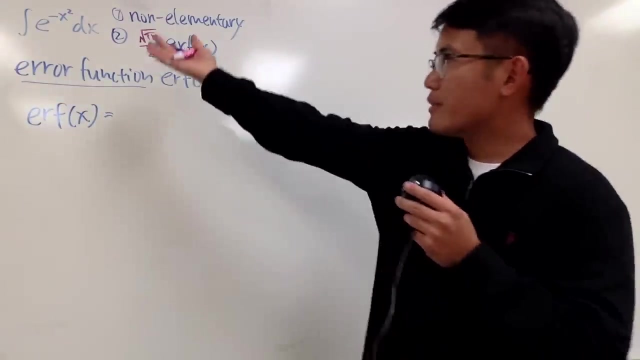 First of all, this is called the error function And once again, I will just call this to be the erf f of x. The official definition is that erf of x is defined to be: yes, you have to talk about the integral, so I will have the integral from 0 to x. 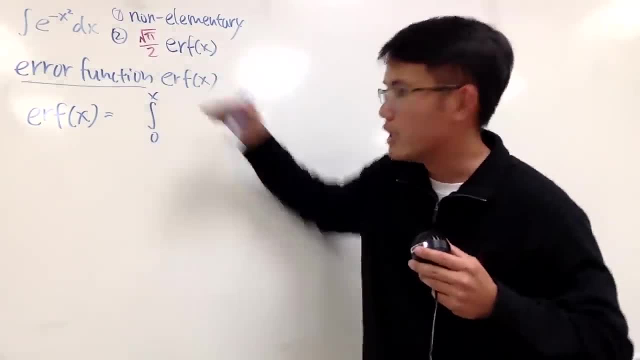 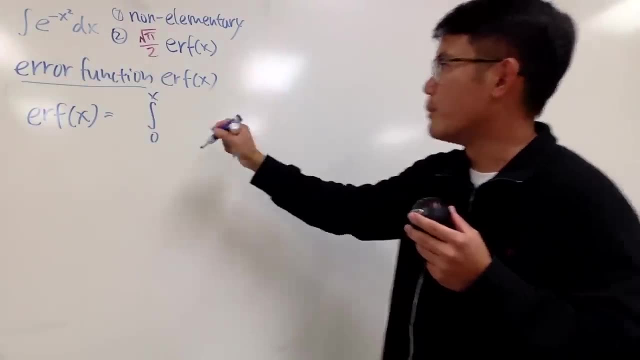 Because the input here is x, I want this to be x as well. This right here is my variable. But if I use x right here, I cannot use x right here to be technical. So just change the variable. let's say t e to the negative, t squared, and then we just put down. 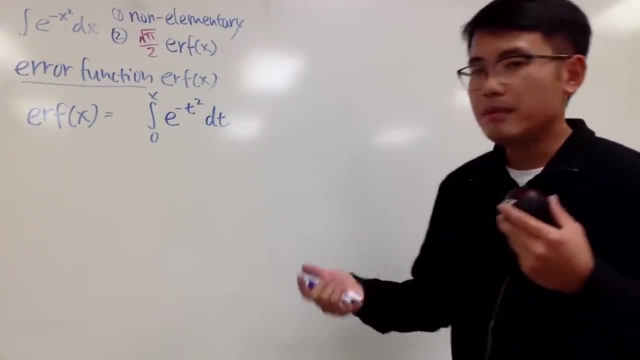 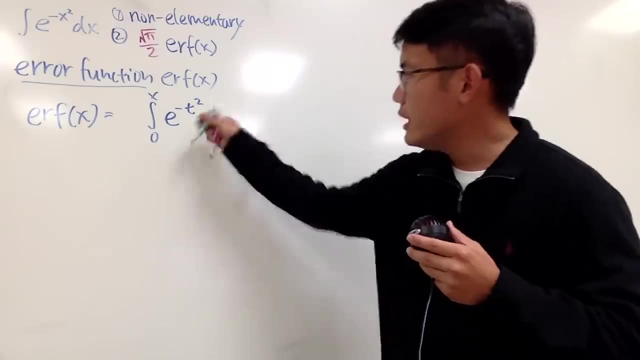 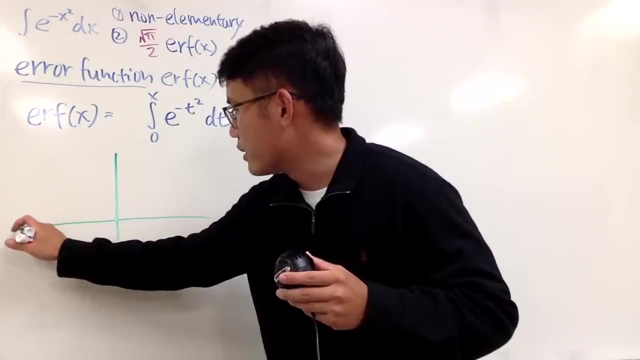 dt right here, But hopefully you guys have seen my previous video. If you guys look at this curve right here and let me just draw that for you guys real quick: e to the negative t squared. In my previous video I used x in terms of the curve. 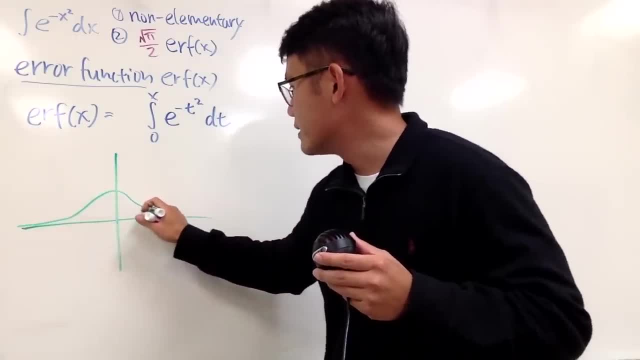 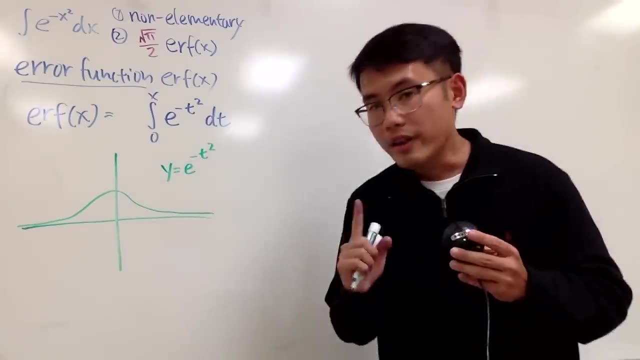 Doesn't really matter, The shape is the same. Looks like this: Okay, So this is the graph of: y equals to e, to the negative t squared, And one of the properties of this is that the whole area under the curve right here. 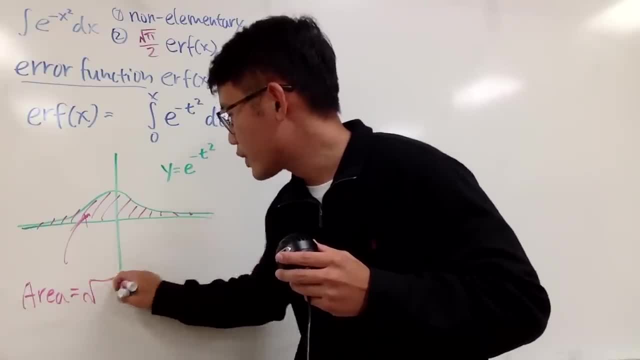 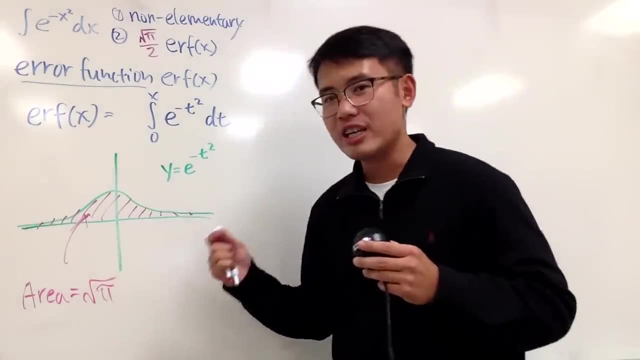 the whole area is, surprisingly, square root of pi. It's square root of pi. Really cool. Once again, if you want to see how to do that, you can check out Dr Payan's video for this. You'll have to use Calculus 3 to show this. 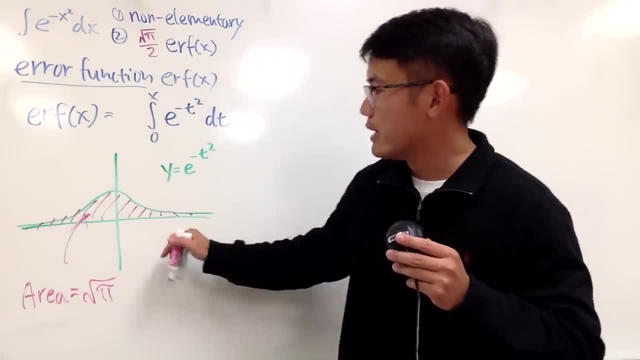 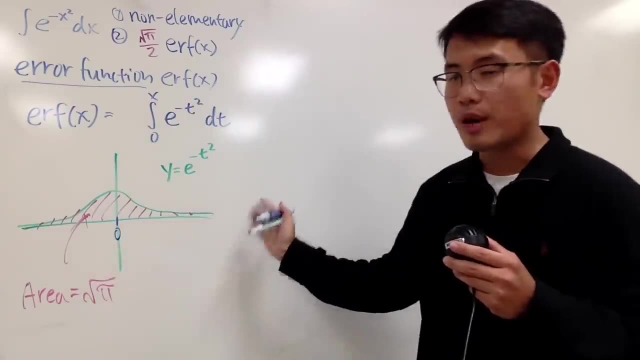 Alright, When you have the integral from 0 to x means that you begin at 0, and then suppose x is positive. then you go, go to the right direction. So you can just say it's right here, And what this is doing is that you are keeping track of the area. 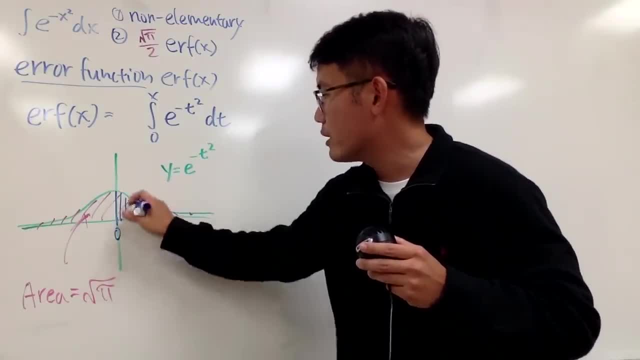 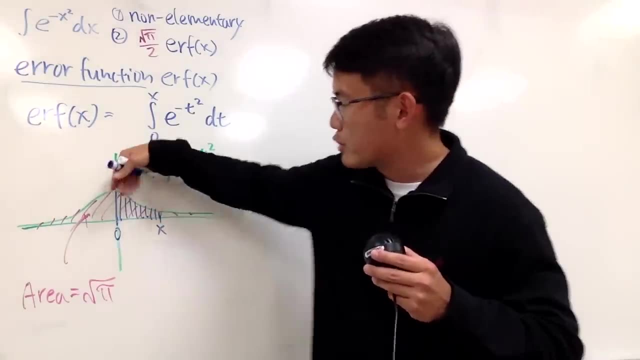 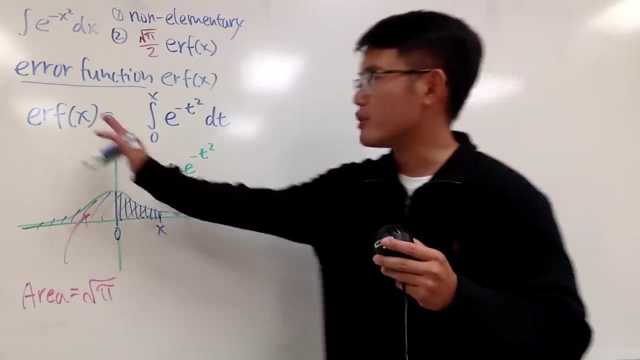 from this part to this part, And this is the blue portion right here. Alright, So this function is pretty much keeping track of the area, But hmm, in statistics what we want is the whole area under the curve to be 1.. 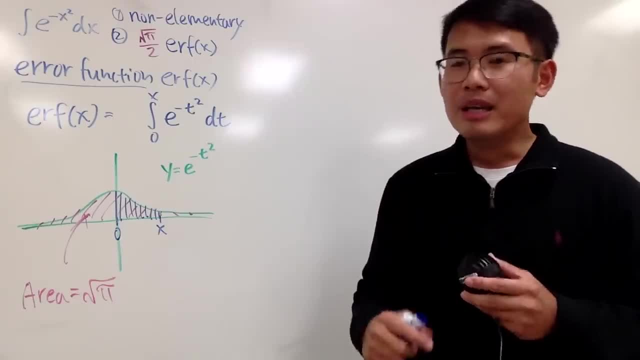 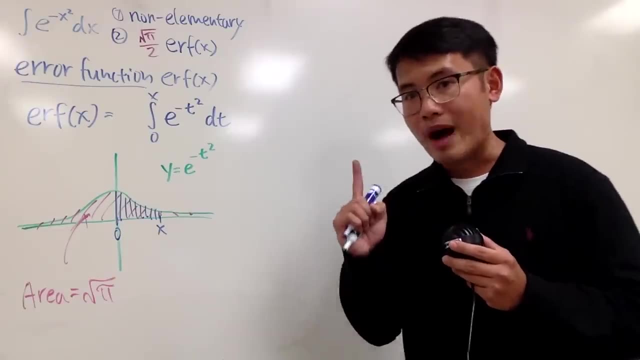 Why? Because what we call the probability density, the probability density function- just a quick example- is that the whole probability is 100% right. That's pretty much the idea. So we want to have 1.. So instead of the whole area being square root of pi, 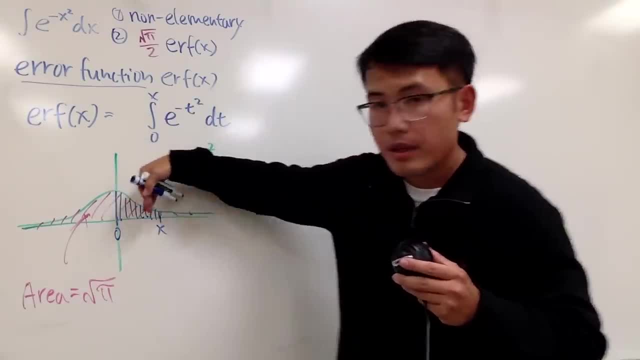 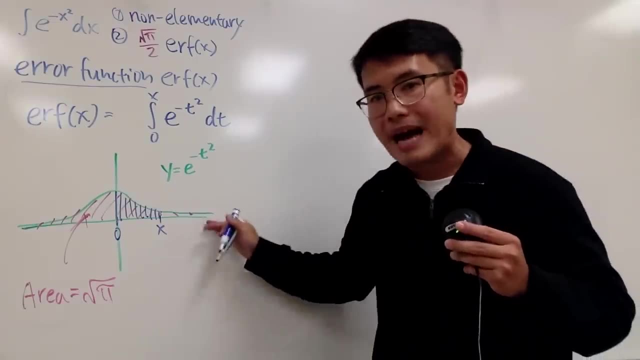 but technically, since I started at 0 to x, if you have x goes to positive infinity. this right portion right here is just square root of pi over 2.. But, as I said, I want to have 1., So I can just multiply by 2, over. 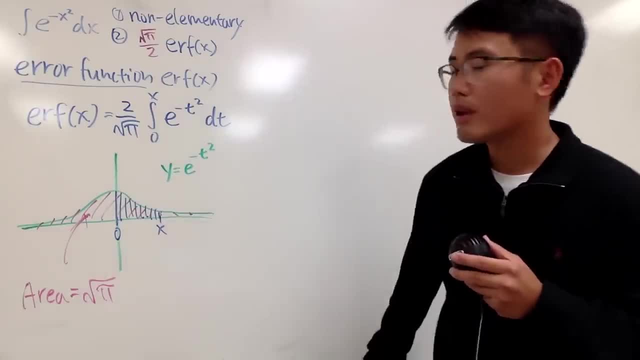 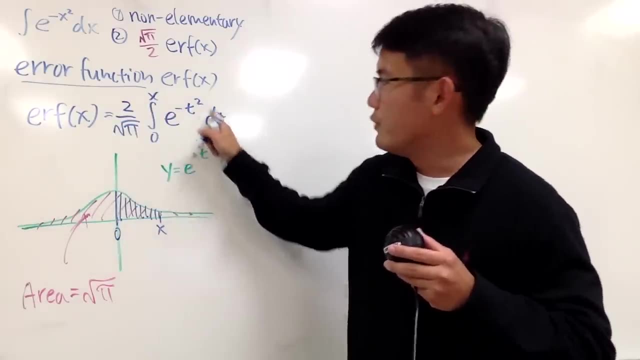 over square root of pi like this, And, as you can see, the area function is defined to be this: If you want to integrate this guy, you can just multiply by the reciprocal, namely you get square root of pi over 2,. 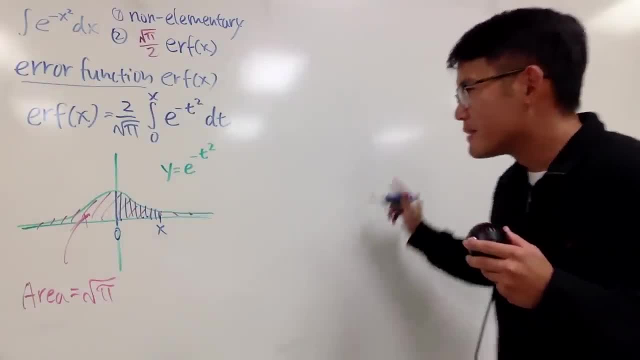 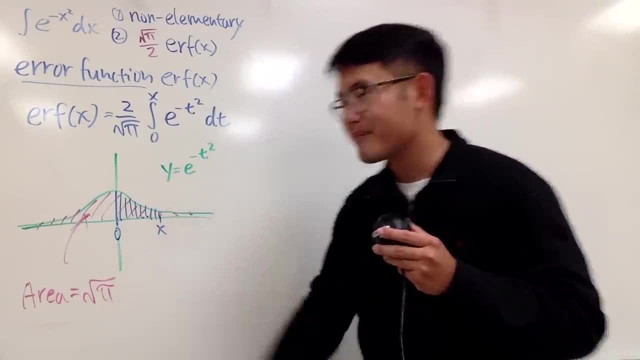 eRf of x for the answer of that. Alright, Okay, And once again, this right here is pretty much a reciprocal of the right hand side area, Alright, So, hmm, this is not. this is not good enough, I know. 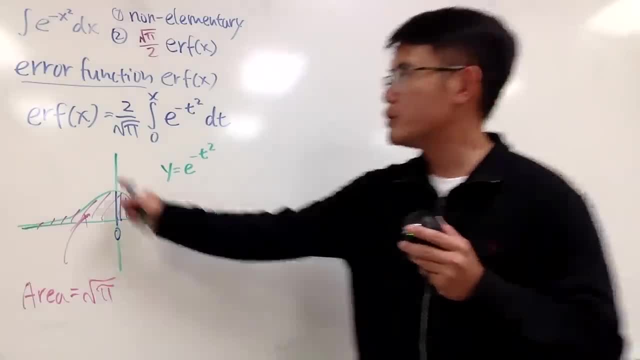 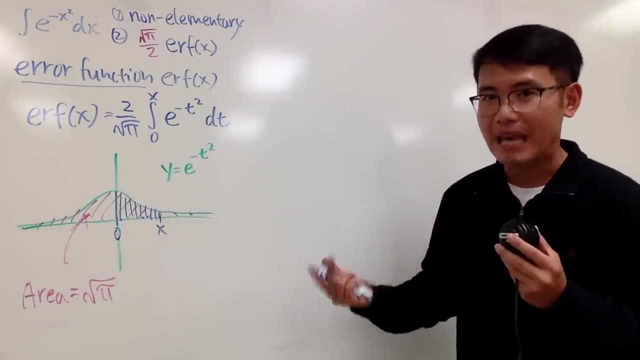 I will do more for you guys. Perhaps the best way is I will show you guys the graph of this function, because graph is one of the best ways to visualize how the function behaves. It gives me so much information, right, But with that being said, we have to do more work as well. 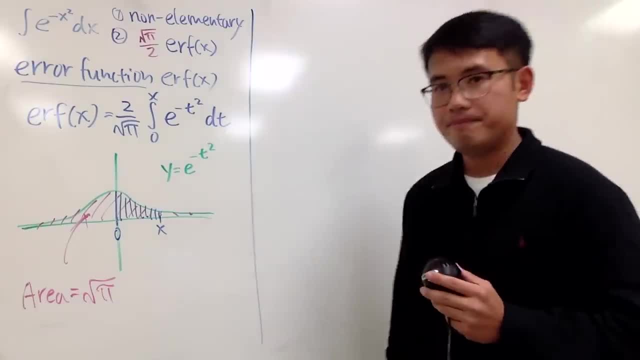 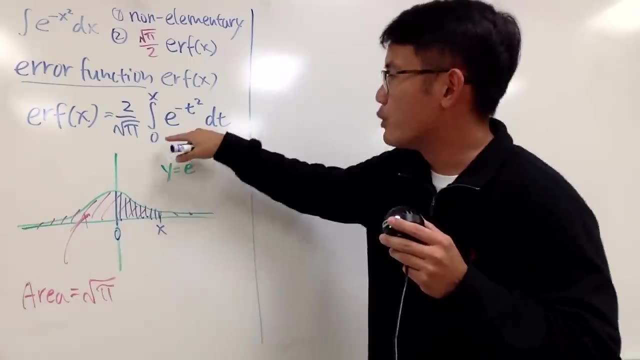 So it's okay, let's do it. First of all, x right here can be positive or negative If you went to the negative side. when you go from 0 to negative, what so ever, you can just flip the integral if you would like. 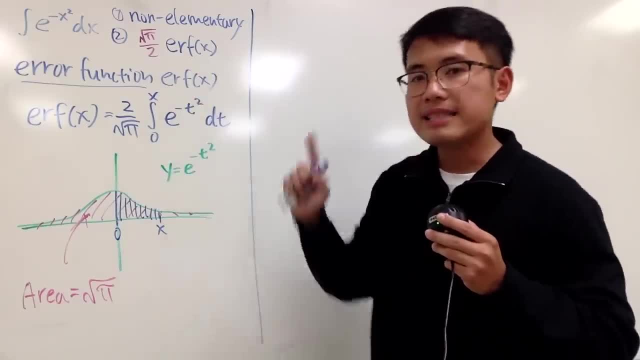 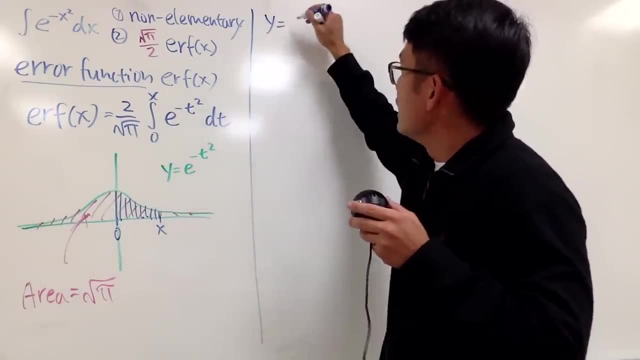 so it doesn't really matter that much, But the main point is that x can be anything for eRf of x. Therefore, if you want to talk about the graph of eRf of x, first of all let's talk about the domain. 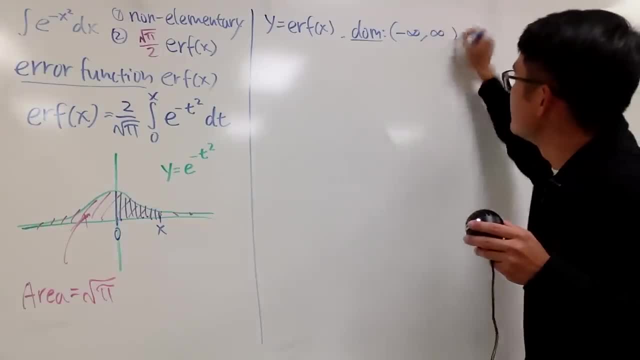 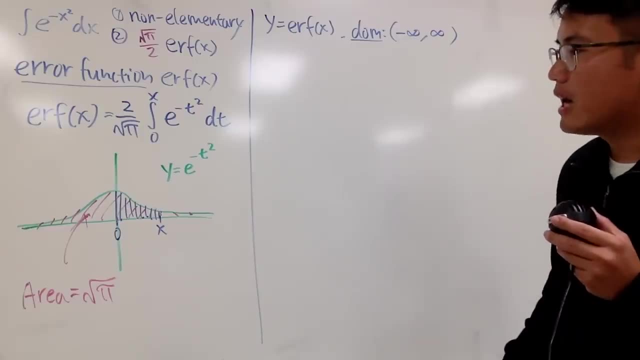 which it will be from negative infinity to positive infinity. Okay, So that's good, We can plug in any x values that we want. And secondly, let's find out the horizontal obstacles. Shall we? Therefore, let's go ahead and take the limit. 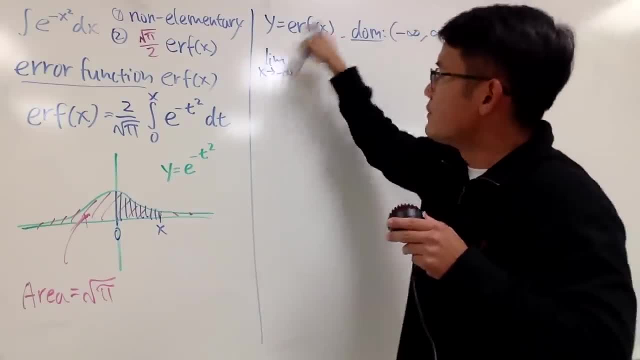 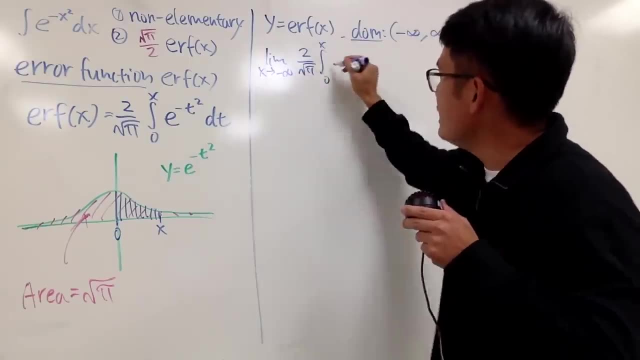 as x goes to negative infinity. first, And for this function let me just put this down: Namely, we have 2 over square root of pi times the integral from 0 to x, And then we have e to the negative t squared dt. 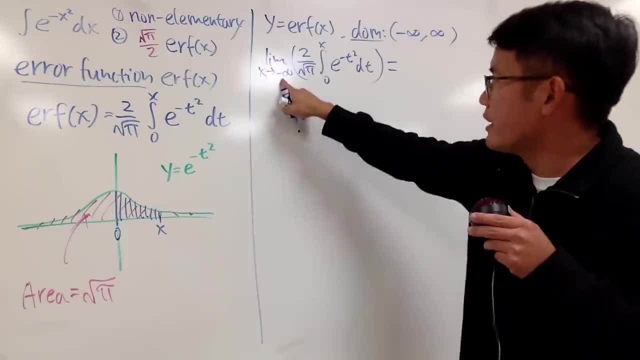 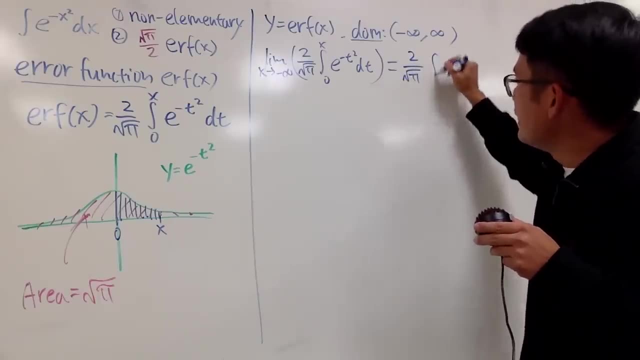 And you see, when you have this right here, you technically can plug in negative infinity to here. This is where the x is. So this is going to look like 2 over square root of pi, integral from 0 to negative infinity. 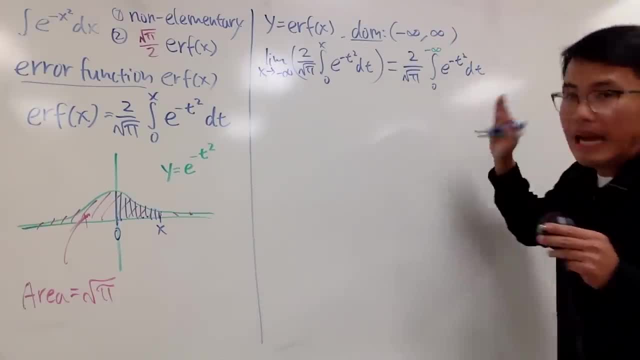 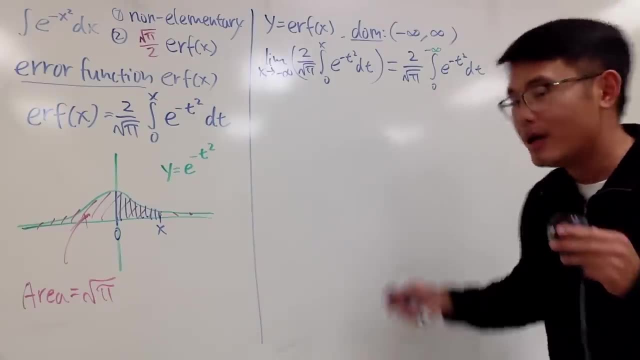 And then this is e to the negative t squared dt. And this, right here, is what I was saying. It's kind of out of order Because right here you should have a smaller number down below, But you have negative infinity right here. 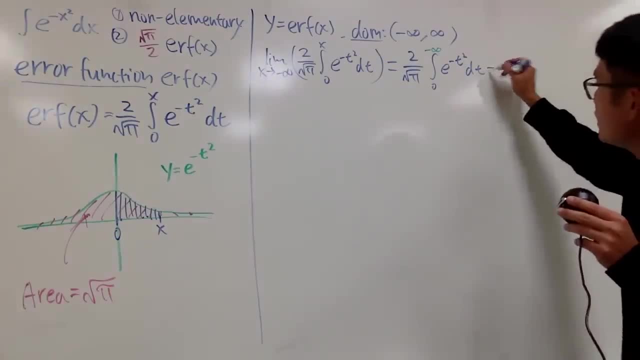 That's no good, But it's okay. It's an easy fix. What we are going to do is I'm going to multiply by negative and then flip this order. That's pretty much it, So I will still keep this. 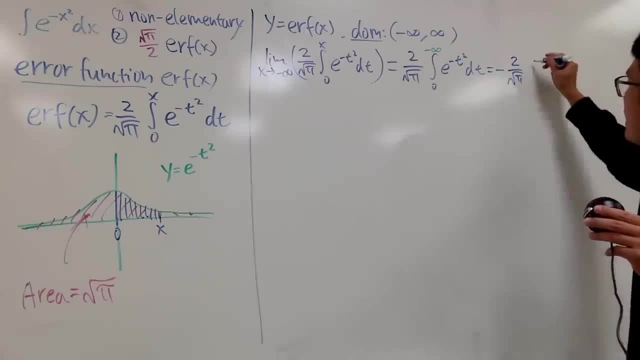 This is 2 over square root of pi And I flip the order, It becomes the integral from negative infinity to 0 of this of course, e to the negative t squared dt. Ah, what's this right here? If you look at this picture. 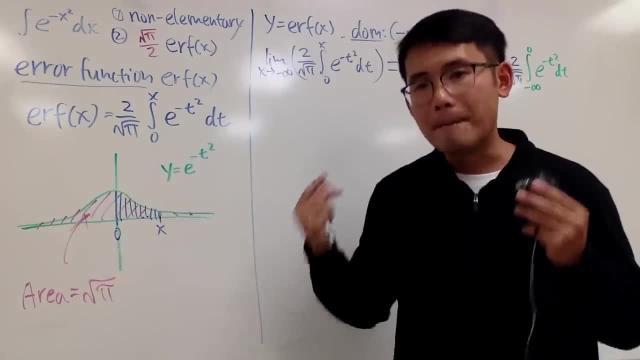 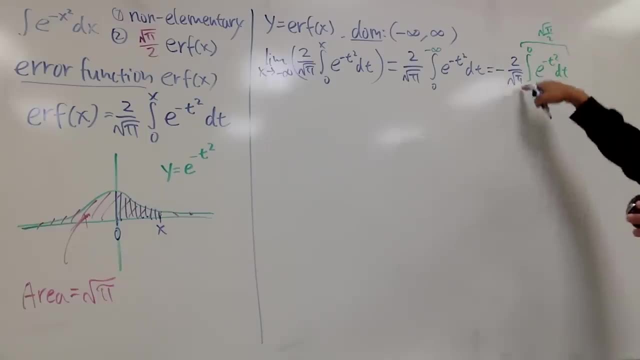 when you go from negative infinity to 0, this right here is still square root of pi over 2.. So this right here is still square root of pi over 2.. Multiply by 2 over square root of pi, you get negative 1.. 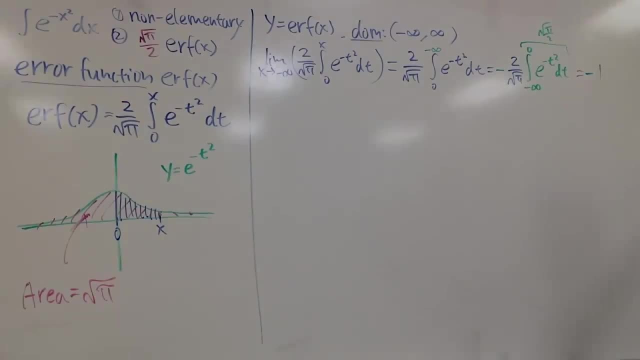 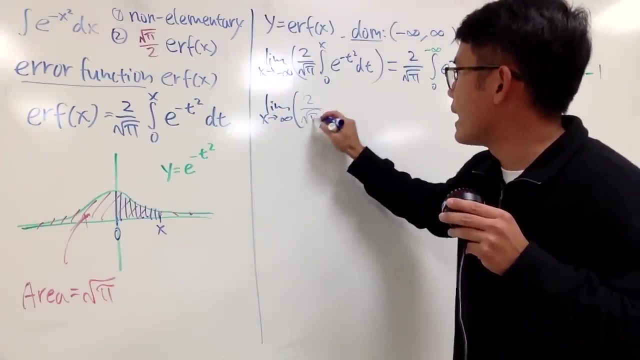 So you have the first horizontal asymptote at y equals to negative 1.. And if you take the limit as x goes to positive infinity, of this, 2 over square root of pi- and in fact you know this right here- is actually an odd function. 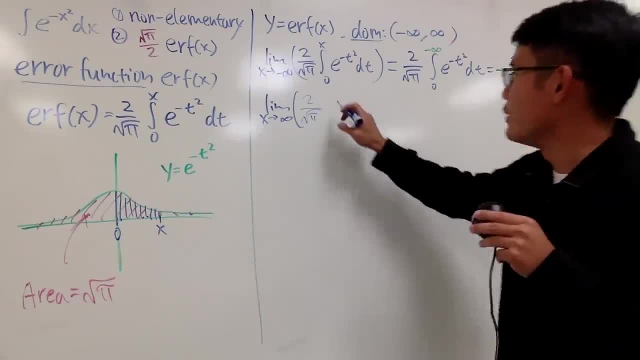 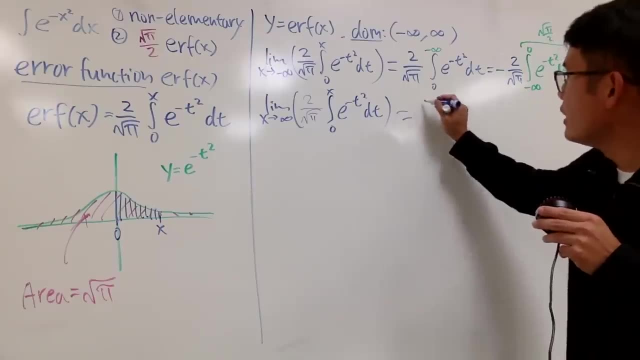 so the answer is going to be positive: 1.. But it's okay, I'll show you guys this right here anyway. This right here is going from 0 to x, e to the negative, t, squared dt, And of course you plug in infinity here. 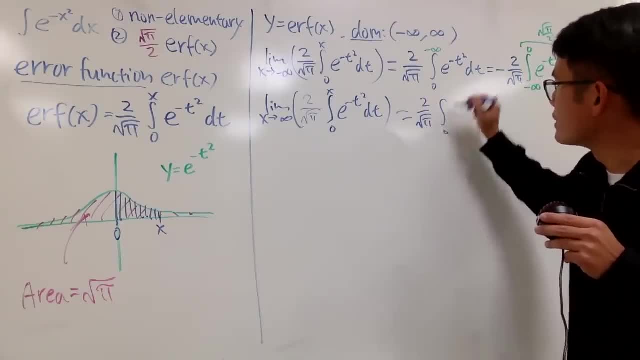 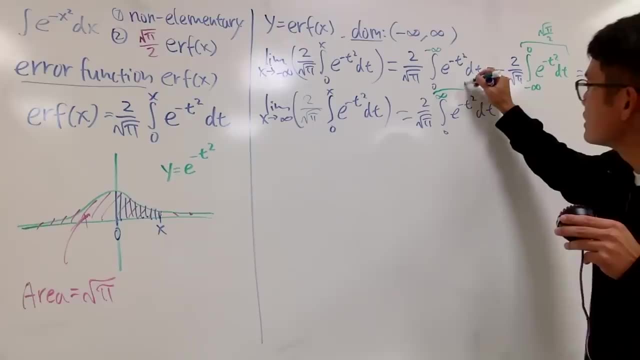 you get 2 over square root of pi and you have the integral from 0 to infinity here. and then you have e to the negative, t squared dt, And this right here is just square root of pi over 2, which is going to give you 1.. 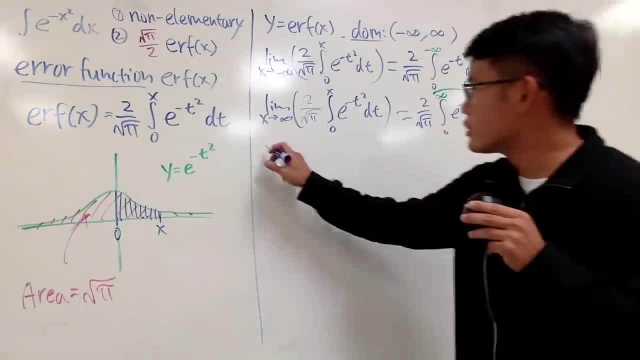 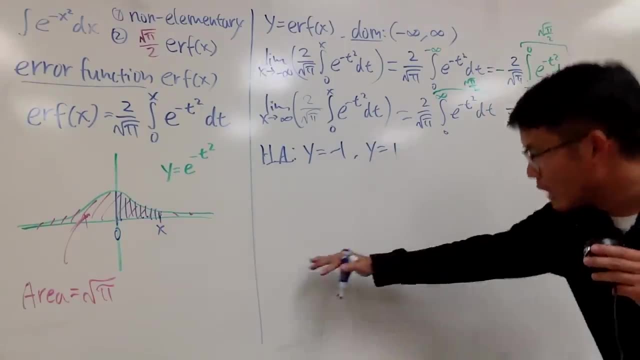 In fact you have 2 horizontal asymptotes. So let me just write down horizontal asymptotes based on our computations You have: y is equal to negative 1, and the other one is y is equal to 1.. So you have these boundaries, okay. 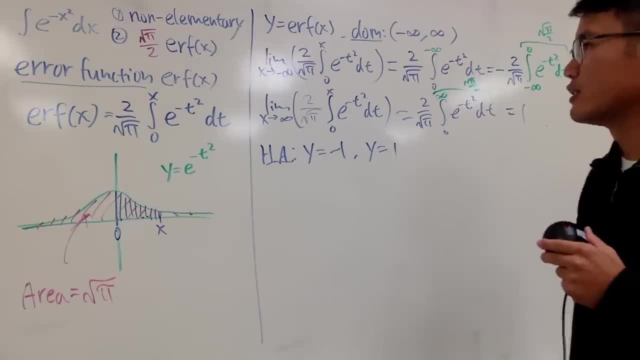 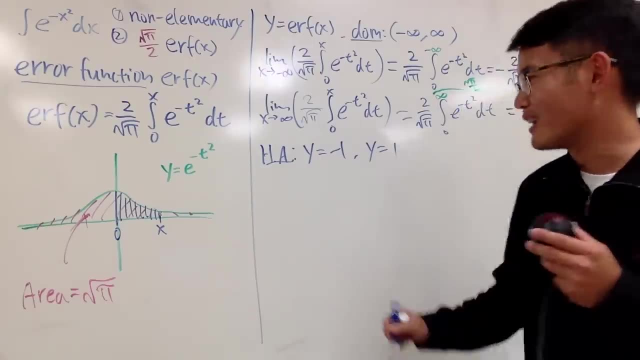 And now let's see if there's any vertical asymptotes. But since the domain was all real numbers, so there's none. And let's talk about first derivative. This is the fun part. Let's see. I will look at the function. 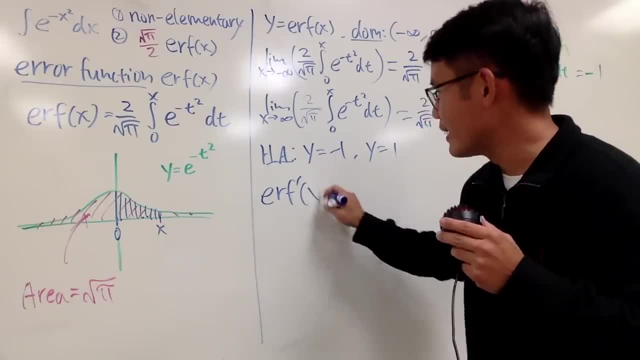 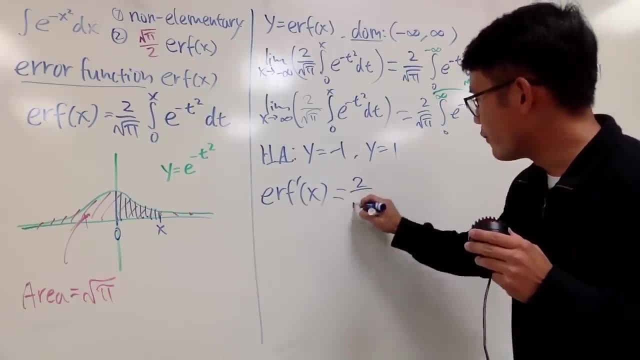 I will just write down erf: prime of x. How do we differentiate this function? This is just a constant multiple, so you just leave it 2 over square root of pi and by the fundamental theorem of calculus, part 1.. All right, 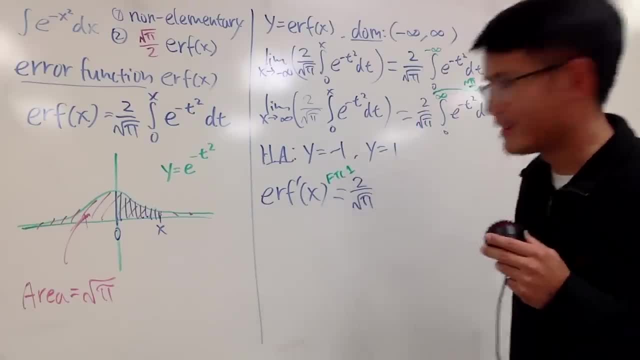 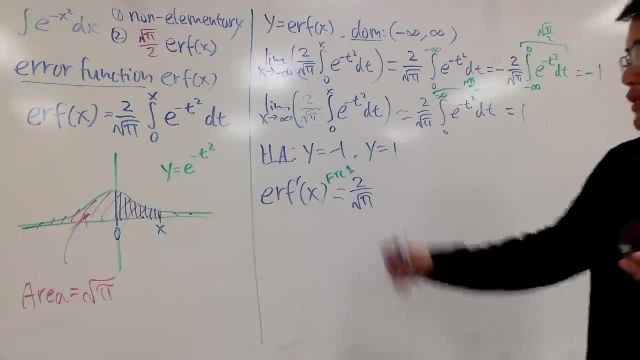 So I will tell you ftc part 1, okay, All you have to do is put the x right here. That's it, And the derivative integrals pretty much cancel this shadow. and you put the x right here, So you get e to the negative, x squared like this: 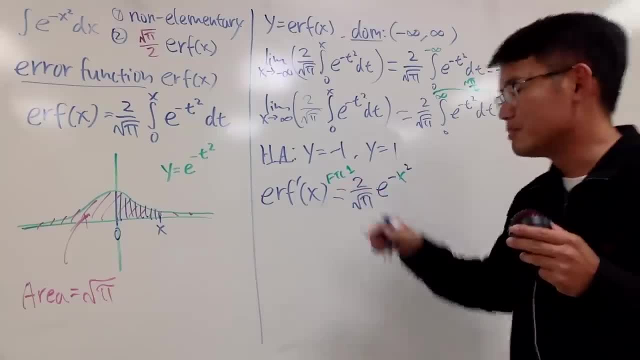 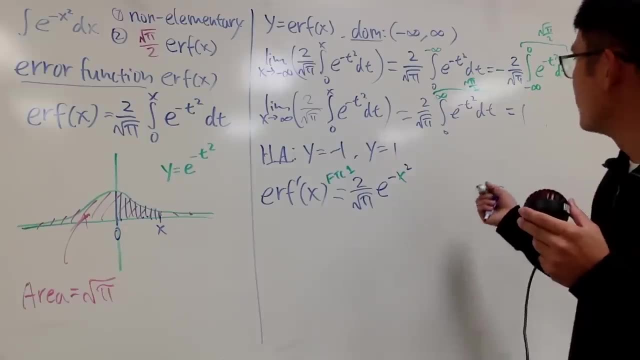 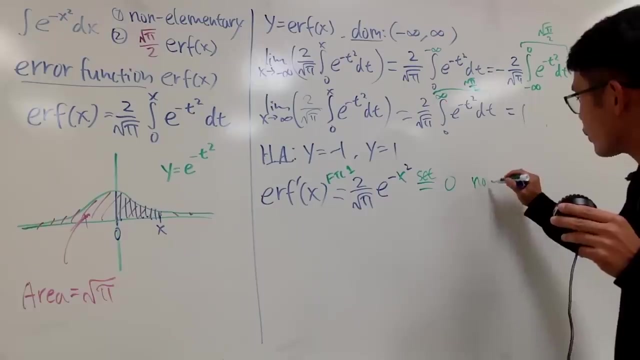 That's it Seriously. it's just that easy. This is my favorite calculus 1 question And if you look at this and perhaps you can do what we did last time, if you set this to be 0, well, you don't have any critical numbers. 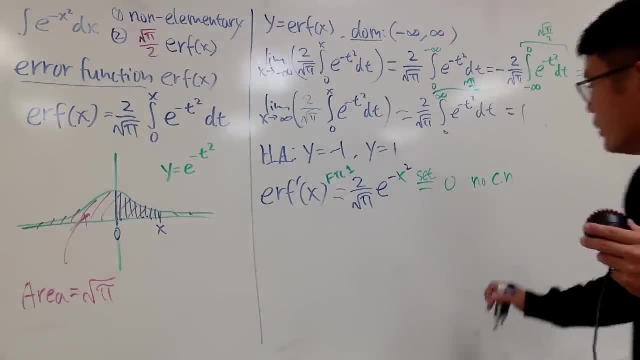 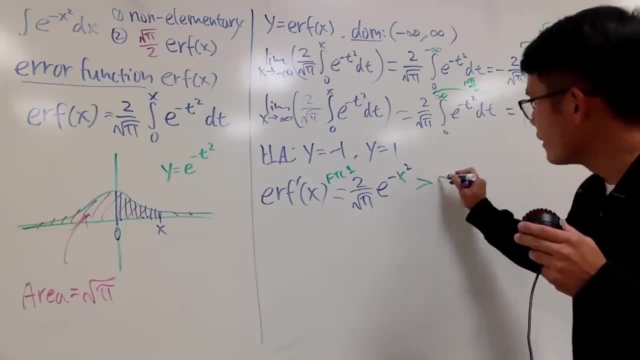 So I will just tell you no critical numbers. And in fact this right here is never 0. And you can actually say more. This right here is actually always greater than 0. And with this we can say that this function is always increasing. 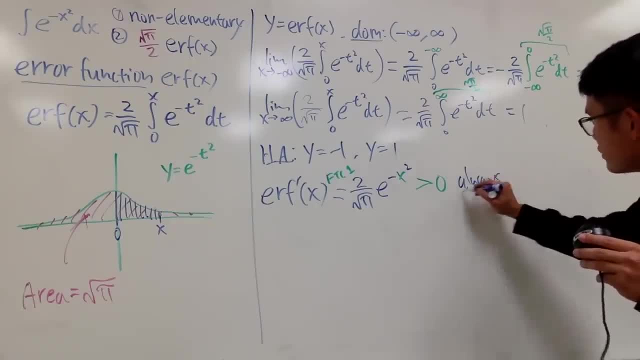 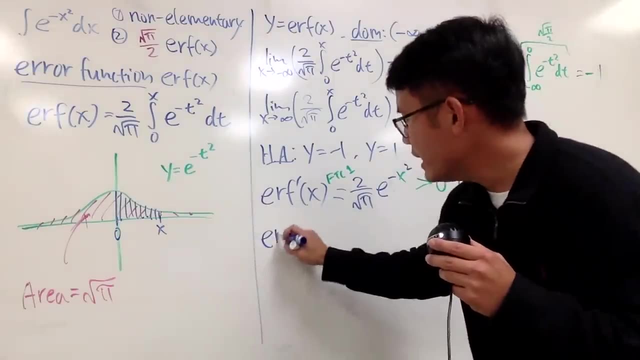 So let me just write this down: The error function is actually always increasing. And now let's move on to the second derivative. So I will look at this and differentiate and I'll write down er f, prime, prime of x, like this: Well, all I have to do is look at this and differentiate. 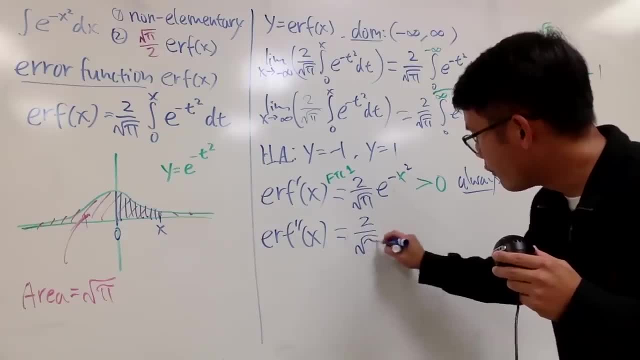 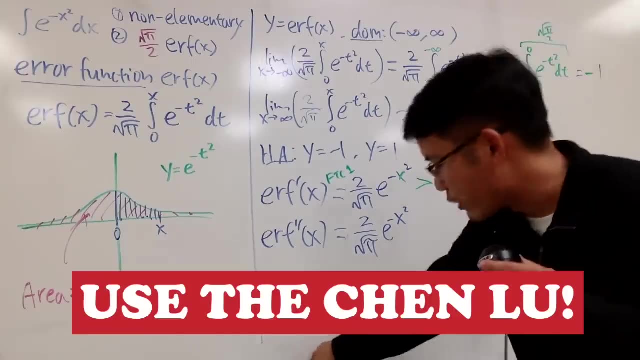 But this is the constant multiple. I can write it down: first 2 over square root of pi And then derivative e to the. something is always that. So e to the negative x squared. But you have to use the chain rule. Use the chain rule. 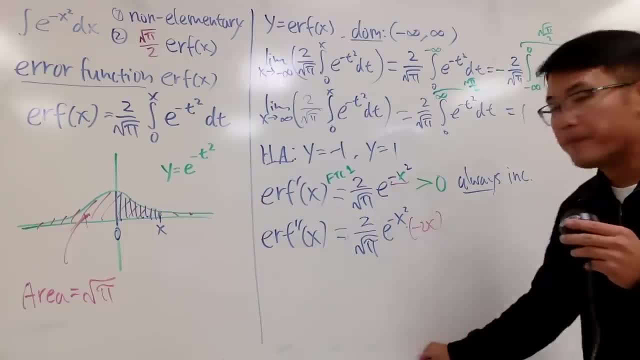 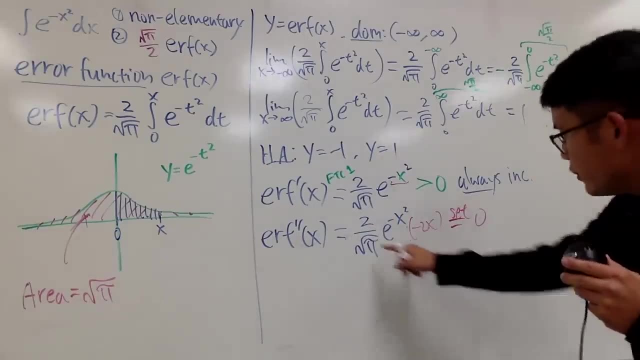 I have to multiply by the derivative of that which is negative, 2x, like this, And right here I will set this to be 0 so I can find out the potential point of inflection. And if you look at this, the only way that this can be 0 is when x is equal to 0. 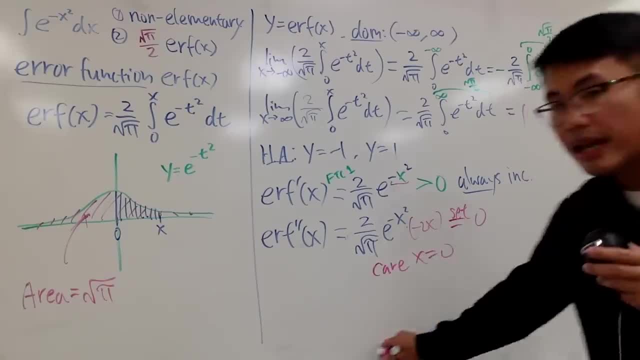 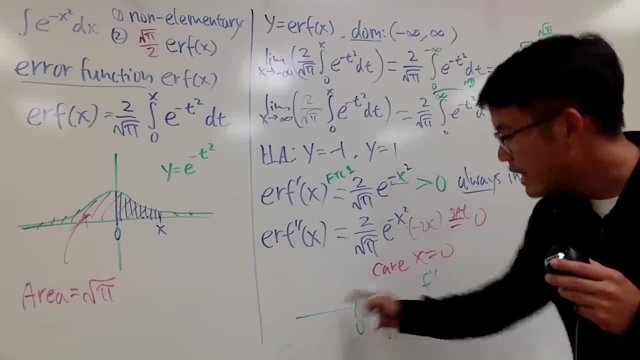 So I will tell you we care about when x is equal to 0.. And then from here we can go ahead and do our second derivative test like this: So I mark it as 0.. And now let's pick a number less than 0.. 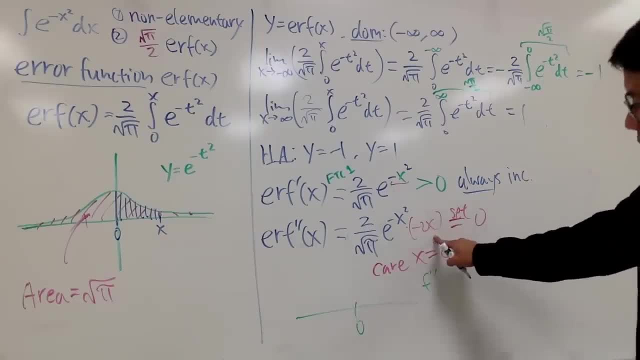 Let's say negative 17.. Plug into derivative Here: negative 2 times negative, 17 is positive Times, the rest is positive. So right, here is positive. And then pick a number bigger than 0. Let's say 25.. 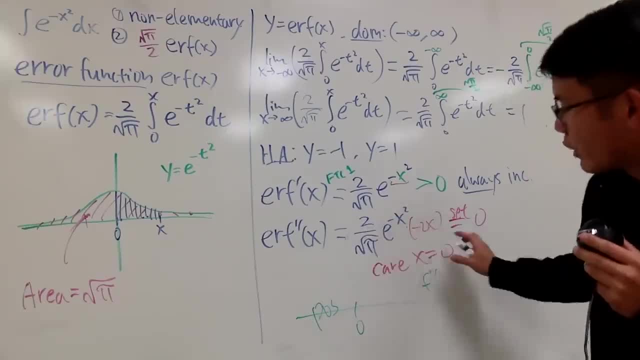 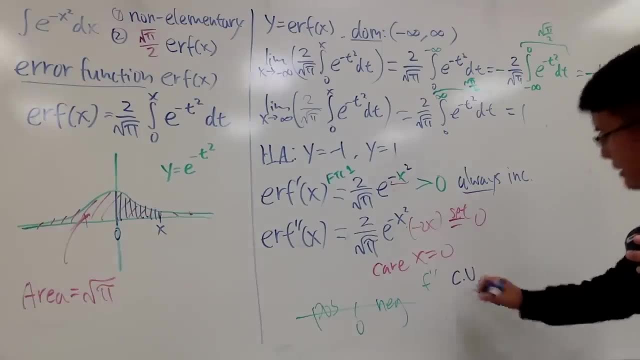 Plug into here. Negative 2 times 25 is negative Times, the rest is positive, So altogether it's still negative. This right here is negative. So what does that mean? This right here tells me: concave up. Cu stands for concave up. 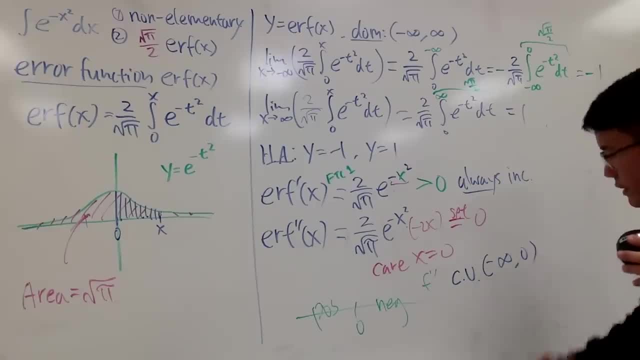 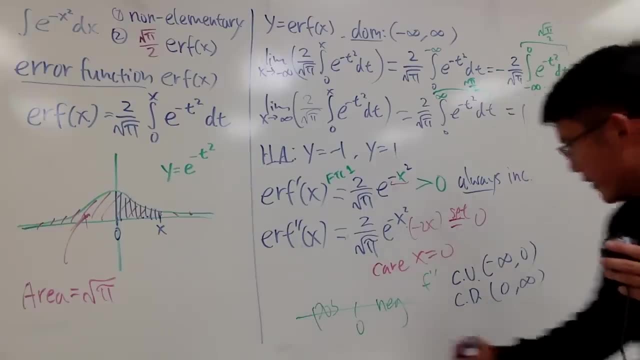 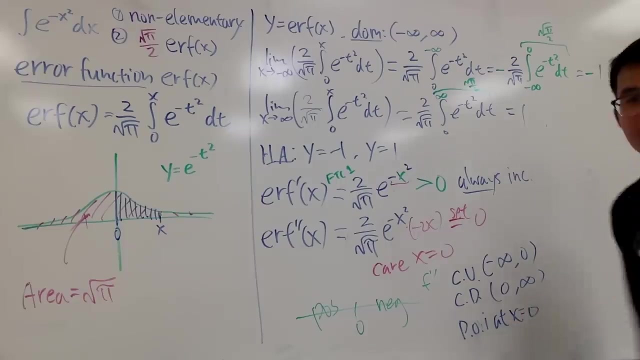 From negative infinity to 0. And then concave down. So I put on Cd like this: From 0 to positive infinity. And then we do have a point of inflection. So I put on Poi like this: Add x equal to 0. 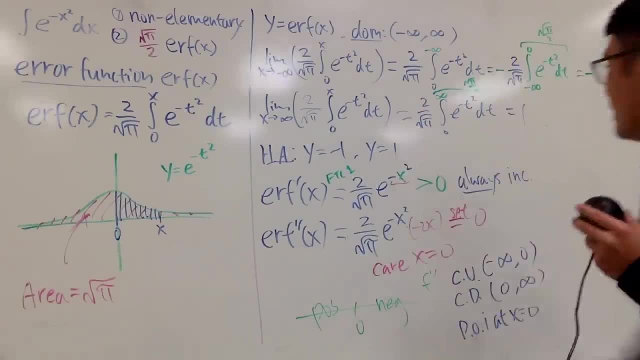 So now, in fact, with all this, I can show you guys the graph And I will do the graph right here And I'll show you guys the graph on the screen. So I'll just put this down right here. I know it's a small one, but it's okay. 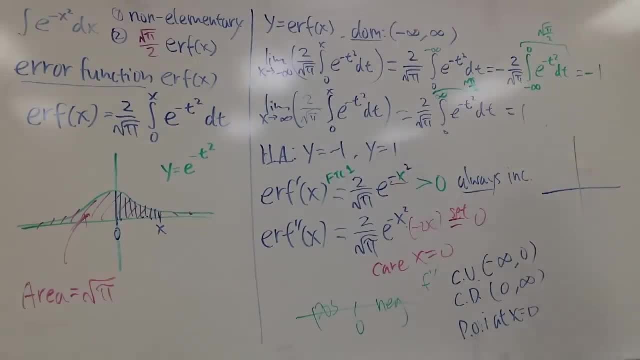 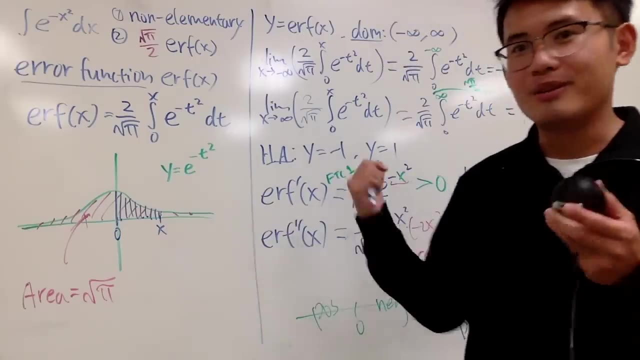 First of all, domain is all real numbers And let's see, Everything is increasing And perhaps you can find out some like: seriously, just pass some numbers So you can know where to grab this. Put 0 into here, You get Erf of 0. 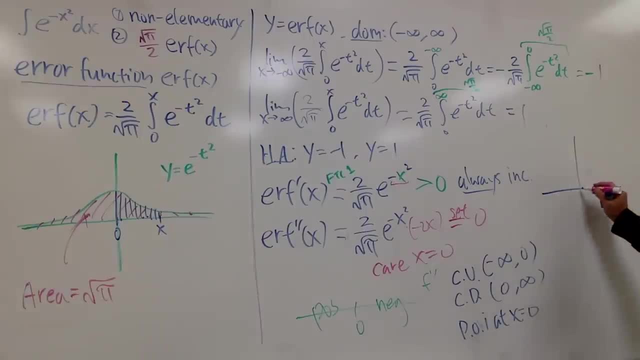 You put 0 here, 0 to 0. You get 0. So you have 0 right here. And let's see, We have the horizontal asymptotes. Let's indicate this: We have negative 1.. And then we have positive 1..